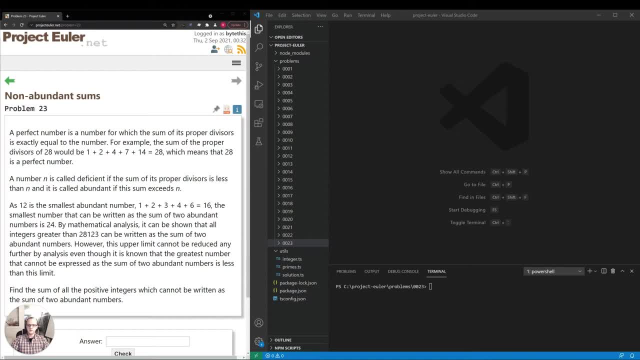 expressed as the sum of two abundant numbers is less than this limit. Find the sum of all positive integers which cannot be written as the sum of two abundant numbers. Okay, so this one has an interesting premise in the middle. there They state: it can be shown that all integers greater. 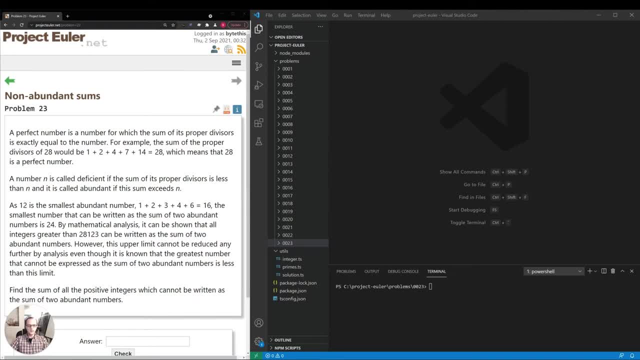 than 28,123 can be written as the sum of two abundant numbers. but they say they know that the greatest number that cannot be expressed is less than n. They just can't seem to prove it by mathematical analysis. So it looks like we'll be able to prove. 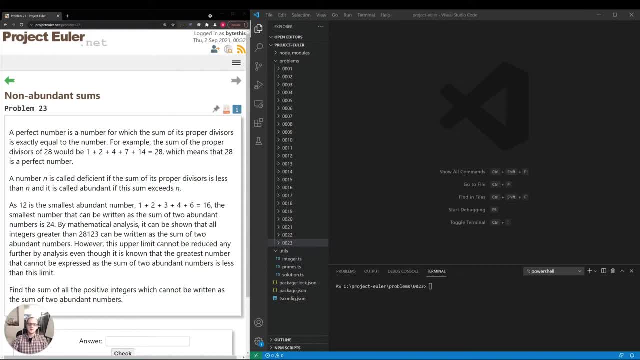 it ourselves today just by computing the solution. but it's interesting that they can't come to the solution based on, as they say, mathematical analysis alone. So let's think about how we want to approach this. So the brute force solution would be to just figure out all of the numbers. 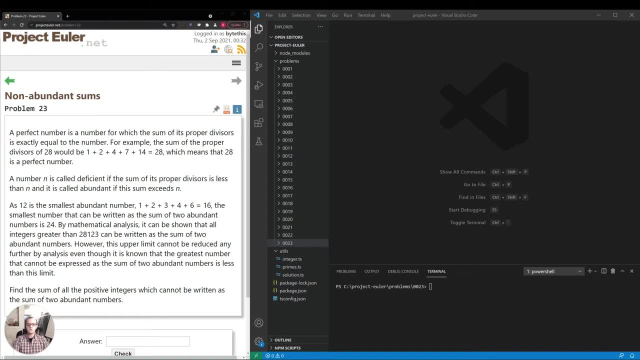 which are abundant by iterating all the numbers 1 up to this 28,123, and if it is abundant then we can add it to some sum value. So we'd have to not only get the factors for each number but then add the factors together. So that's a lot of work. 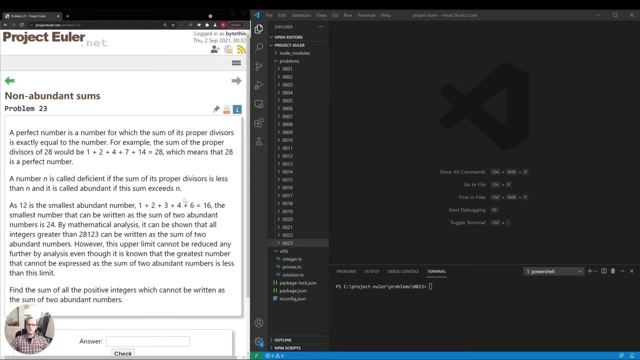 and, I think, a lot of redundant work, because let's take this example of 12.. So if 12 is an abundant number, then I think it would follow that 24 would be an abundant number, because 16 plus 12 is 30. So 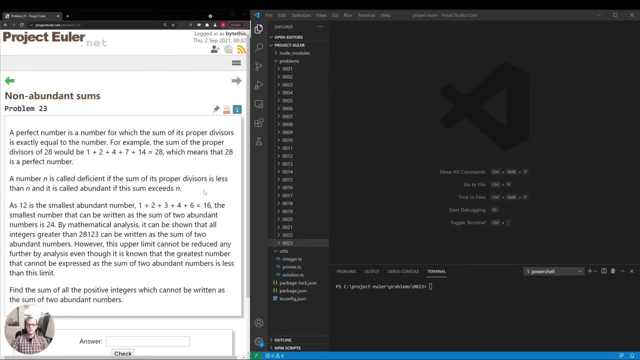 I think we can say that for any number n, which is an abundant number, any multiple m of n will also be an abundant number. So I think we can optimize this by, as we go, removing sets of numbers that we know for a fact will be a number number. 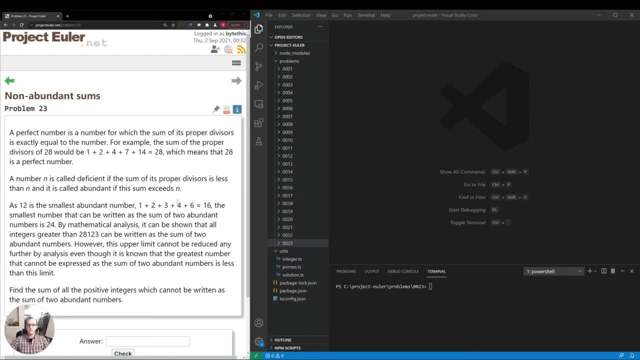 abundant. So, for example, in that situation we could remove 12,, 24,, 36,, 48, etc. etc. And continuing on we could do a similar approach. So let's go ahead with that in mind and start. 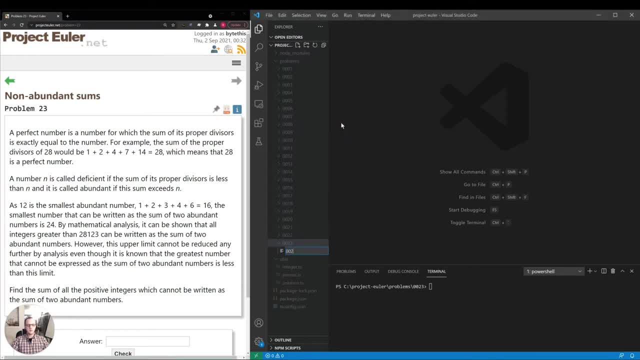 coding. I'm going to be doing this in TypeScript. If you're not familiar with TypeScript, it's an extension of JavaScript And the syntax is very easy to follow along, So you should have no problems following along during the video. I'm going to be coding this in a class which is not 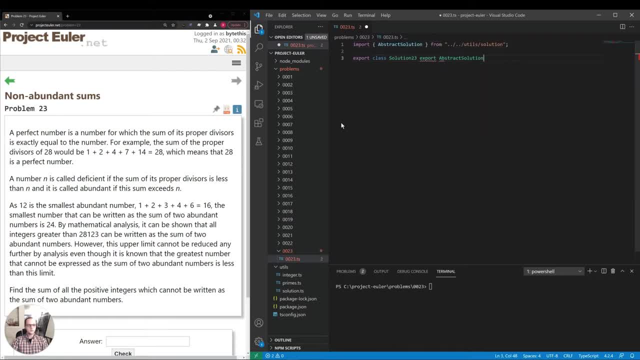 required. I just want to take advantage of some utilities which I've written to run the solution. Okay, so let's go ahead and implement this. The first thing I'm going to do is implement a method which will just tell us if a number itself is abundant. So let's say, private is abundant. 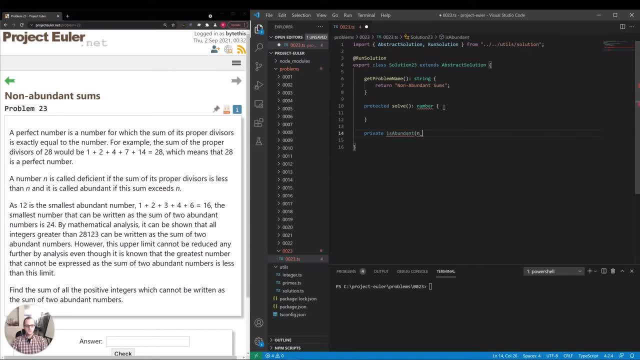 and returns boolean. So let's say first we'll get the factors. So for that we can reuse an implementation we created in a previous video. this integers class. we can just call the method get And then we can just call the method get, And then we can just call the method get And. 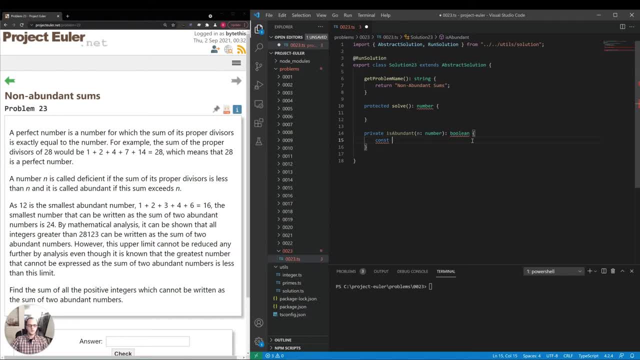 get factors from the class we created and leverage it that way. So we'll say: factors is equal to new integer n dot get. we're going to let's start with get unique factors. So, for example, the number 36, we won't add six twice, six times 636.. So we won't add six twice. So we'll start that way, That's how. 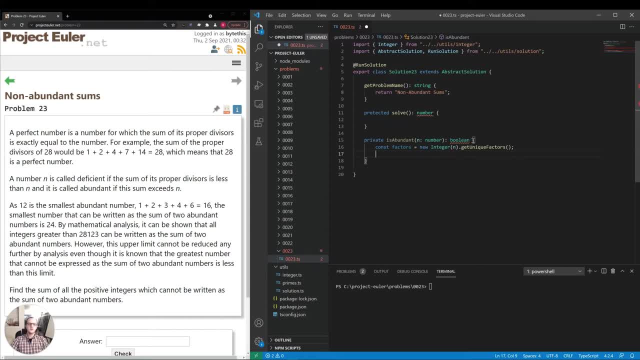 these problems have generally been going. So we have the factors. So what do we need to do now? we need to add them up, exclude the factor which is n itself, So factor sum as equal to factors that reduce accumulator int. So we'll start this with zero And we will return. 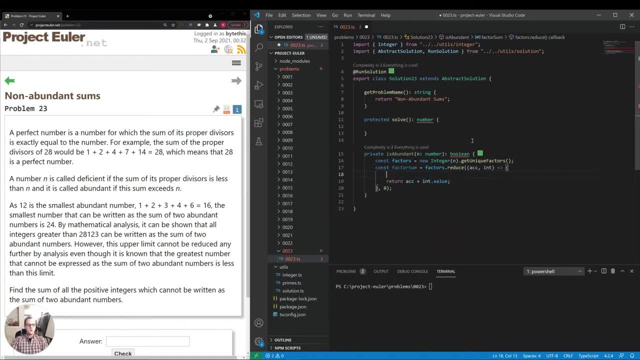 accumulator plus in value. we need to make a check. if int dot value is equal to n, just return the accumulator, So that way we don't add the value in itself. Then we need to return. okay, it's factor sum greater than n. 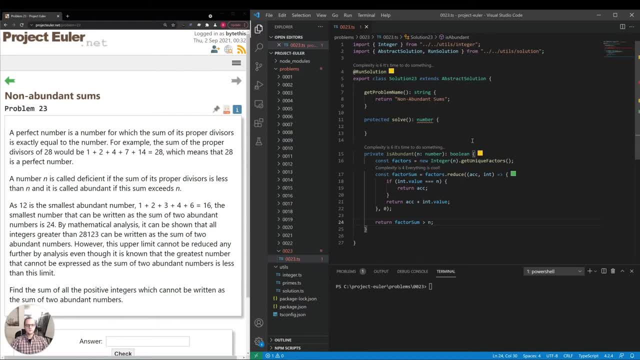 if it is, this thing will turn true. otherwise it will return false. So the question now is: how do we take that optimization and apply it? one thing we can do is make an array of numbers that we know are multiples of abundant numbers So that, for example, we could add 12 to this thing. 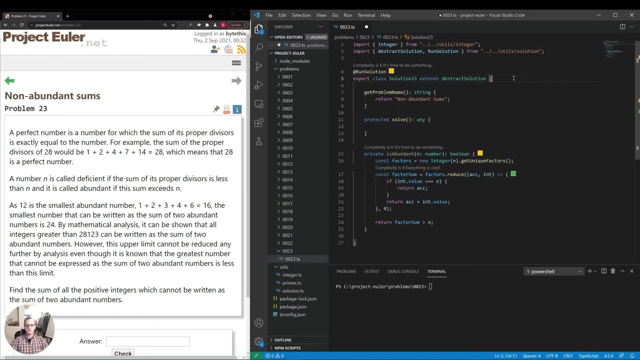 But then I'm thinking at a certain point it's like we're just checking for factors again, like we're not going to have much optimization there. So for now let's just run it without that optimization in mind. we can just check if the number is abundant and go from there. Okay, 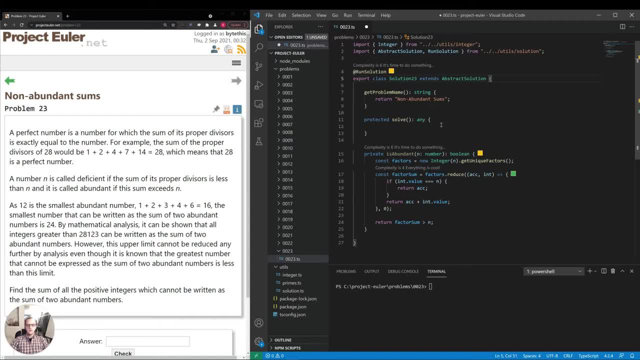 so now that we have the way of determining if a number is abundant, let's check if a number cannot be written as the sum of two abundant numbers. So that part is going to be a little tricky because there's multiple ways to add two numbers together. you get third. 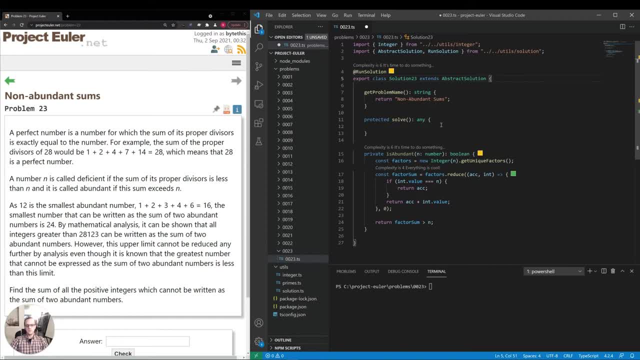 number factor a lot of ways. So if you take the number 1000,, for example, you can have one plus 99,, 999,, two plus 998, etc. So we would have to do a lot of calculation in order to determine if any. 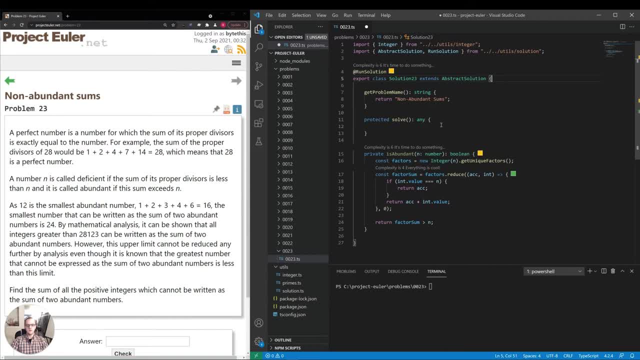 particular number cannot be written as the sum of two abundant numbers. So something we can do at first is just make a list of abundant numbers and then refer to that list when we're checking. So we can say, okay, if our number is 1000,, for example, we can say 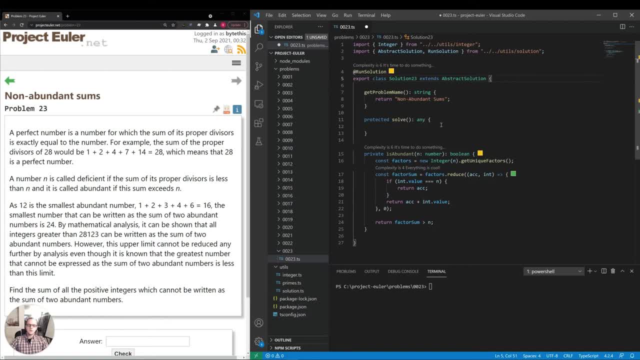 okay, look up. for each abundant number which is under 1000, is there a corresponding abundant number which? that plus this abundant number equals 1000.. So I'm thinking we can use a sorted list for this. So in the last video I installed one of the libraries which I've written, which 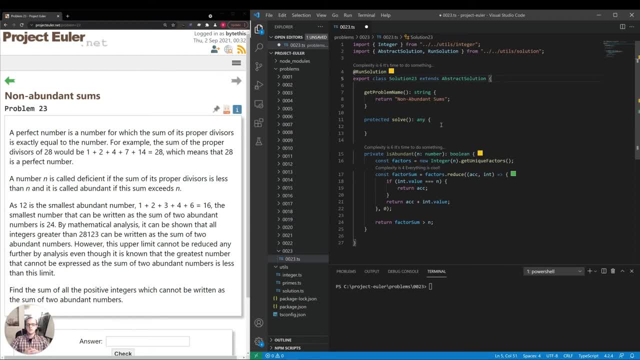 contains a sorted list implementation which, behind the scenes, keeps an array continuously sorted as you add items. So that way when you want to look up something in the array, it will take less time just using a normal array and checking each item. So, to be more specific, uses binary search to check. 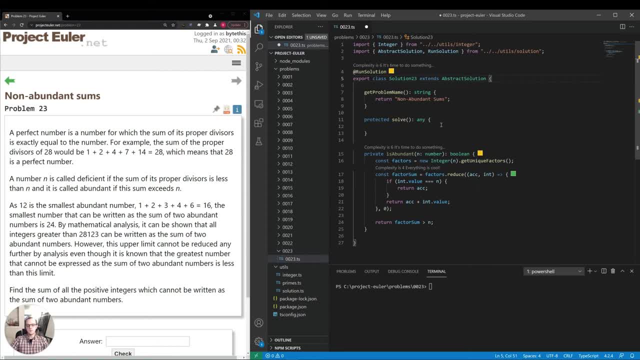 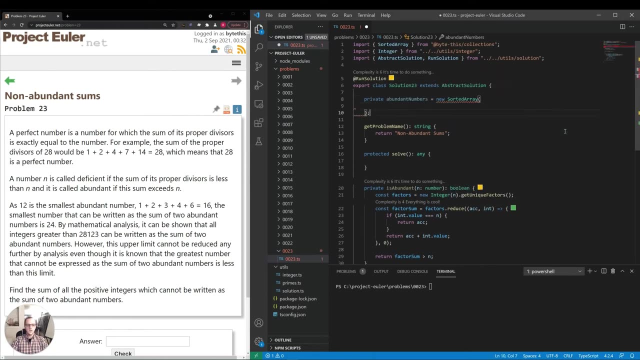 if an array has an item, we're not using a lot less computations than what would normally be done, So let's use that structure. So let's create an array, a sorted list. I'll call it abundant numbers, New sorted list, sorted array, that is, and we're sorting this by number, So I'll pass in. 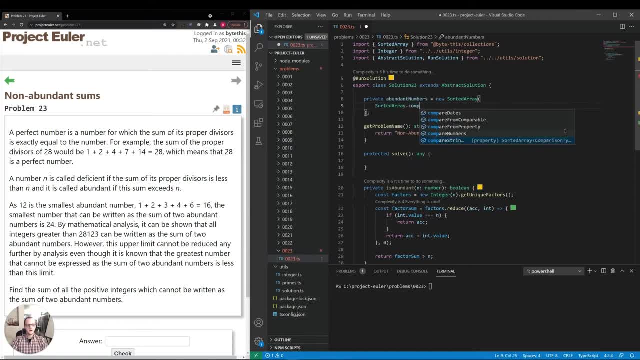 the first argument- sorted array dot, compare numbers- Then I'm thinking, is for each we can iterate from one to 20,123, we can generate all the abundant numbers up to that value, whatever value we're at currently. then do our check to see if two 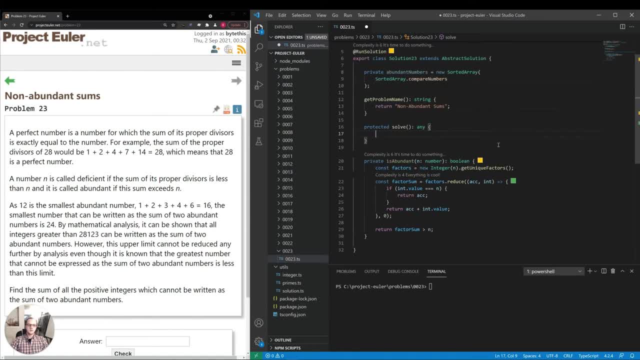 abundant numbers add up to it. So before implementing the rest of this, I just want to do a check on this is abundant, using some of the examples they gave here, And we'll see if the particular number is abundant. So they say 28 is a perfect number, which means that we should get 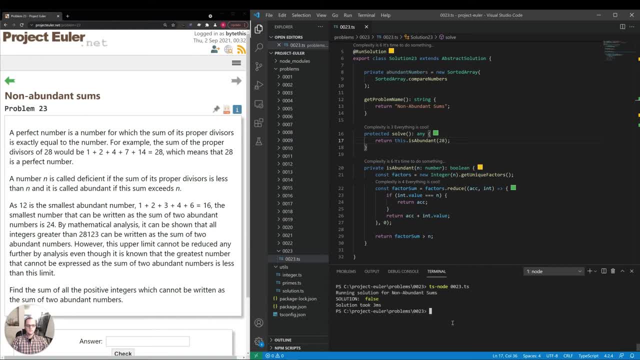 false for that. Good, 12 is the smallest abundant number. we should get true for that. I just want to see what happens if we say the number one itself, Okay, good. So now we have that in place, We'll say for what i is. 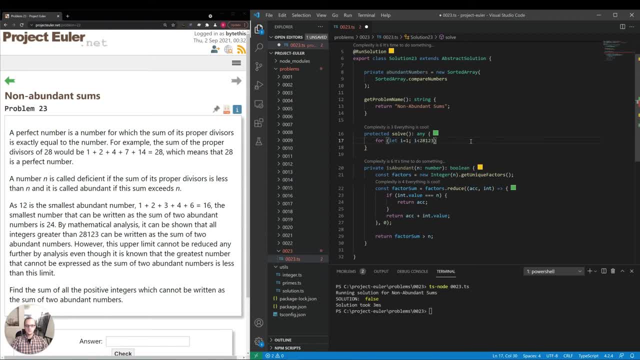 equal to one, i is less than 28,123, 124, because it says greater than 28,123, i plus plus. First we'll say: if this is abundant, I'm going to rename it to end, just for clarity. Now, if n is, 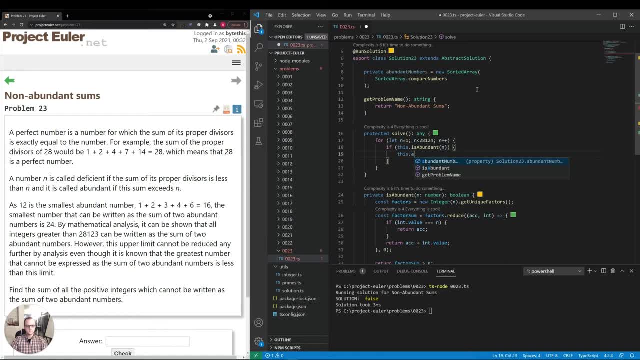 abundant. we're going to add in to our list of abundant numbers. Now what we want to do is take a subset of the abundant numbers between one and n itself. So I'm gonna make a comment here for future iterations, because that won't help us in the current iteration, And then for this iteration, cons. 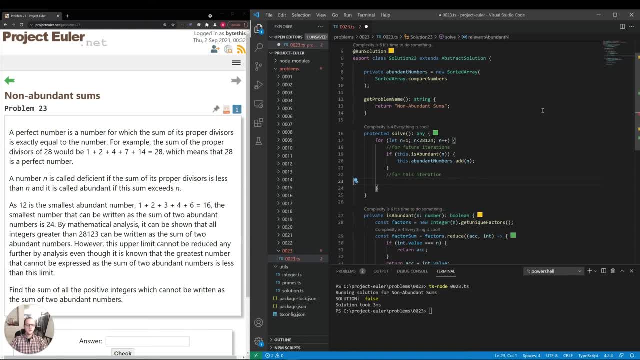 we're going to add in to our list of relevant abundant numbers. Actually, at this point, every number in this array will be less than or equal to n. So what I'll do is this: I'll add that to the end, Then, first, we'll do our other logic. So we want to iterate over the abundant numbers we want. 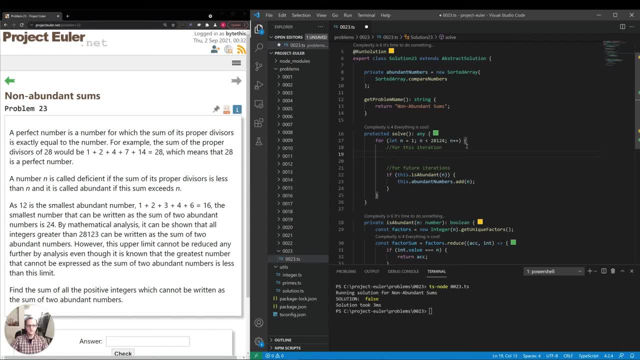 to iterate over half of the abundant numbers and see if there's a corresponding match. So if the number is 1000,, for example, we would want to add in cons that are abundant less than or equal to 500. And then, for each of those numbers, check if 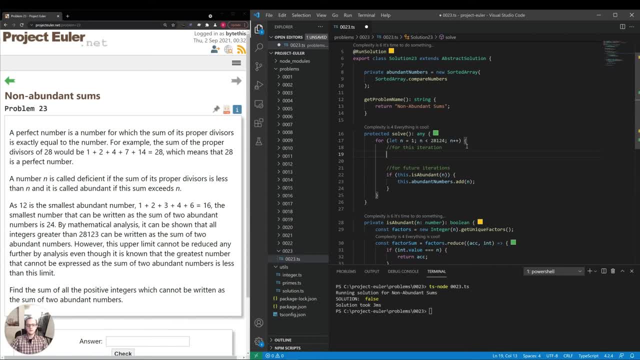 there's a corresponding entry on the other side where that plus a number is equal to 1000. So const sub abundance is equal to this. dot abundant numbers. dot filter Number goes to: number is less than equal to n divided by two. I'm going to extract this part to a separate method. Private is sum of two. 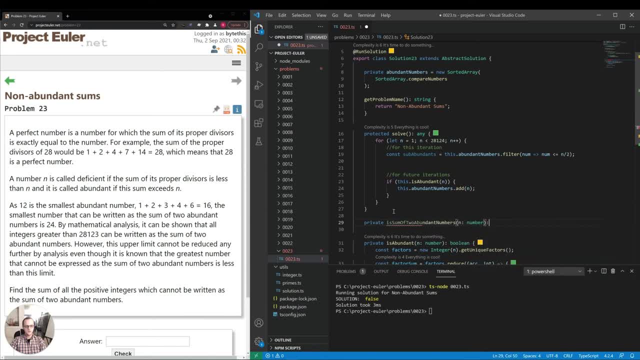 abundant numbers and number or return Boolean. We'll bring this logic in here and then consume it and solve itself. Okay, so we have the sub abundance. then we'll say: for let sub n of sub abundance we're going to check. if we're going to check the abundant numbers, has n minus that number.